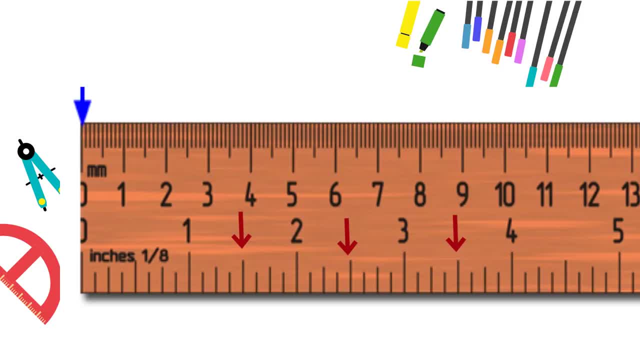 but how did we get this? If you count, you will notice that it is divided into two sections, and if it goes to the half inch mark, you only have one of these. so it is 1 over 2 or one half an inch. This next mark is called a 1 inch mark. The number 2 is the largest mark and if it goes to the 1, 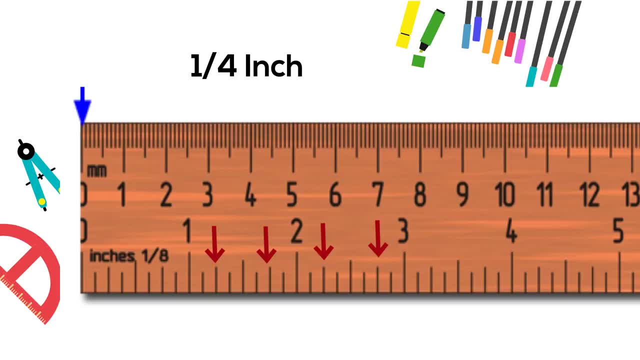 fourth mark- because if you count you have it- divides it into four sections: one, two, three, four and finally, the smallest mark on this ruler divides it into 1, 8th- again you can count- and it divides it into eight equal parts. now let's put this into practice. what is this first measurement? notice it is. 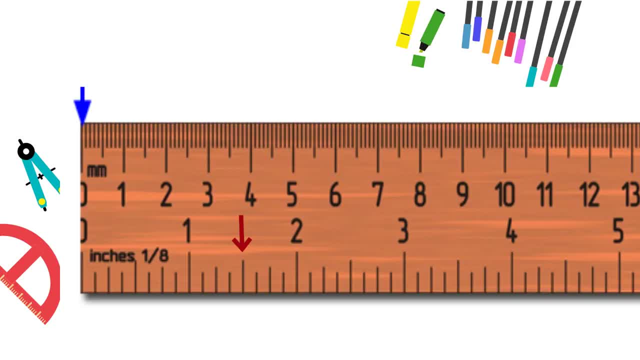 going past the one mark and stops at the one half, so it is one and a half inches. this next one touches the fifth mark of the 1: 8th, so it is one and five eighths. and finally, this one touches the two and one eighth, because it touches the first.